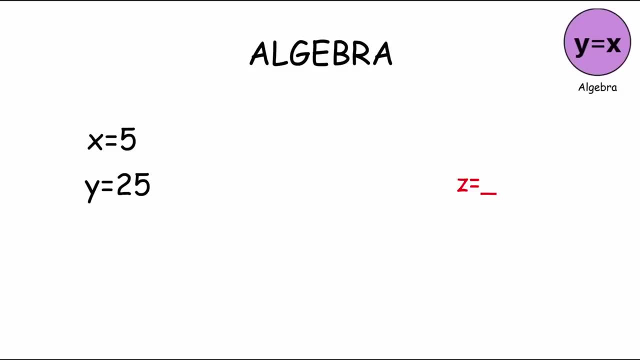 and unknown values in equations. In algebra we work with expressions and equations to understand relationships between numbers and find solutions to various mathematical questions. Geometry- Geometry is a branch of mathematics that explores the properties and relationships of shapes and space. It involves studying angles, lines, circles and other geometries. 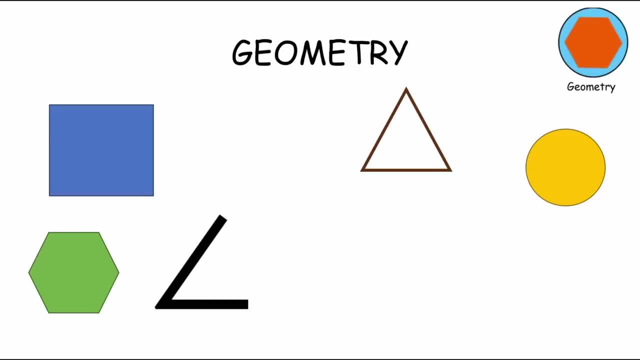 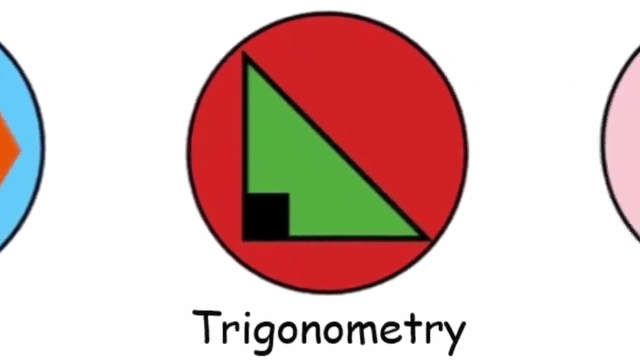 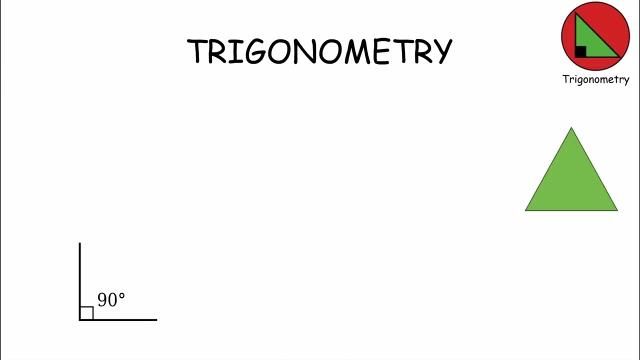 to understand their characteristics and how they fit together. Geometry helps us solve problems related to measurement, design and the spatial effects of the world around us. Trigonometry: Trigonometry is a branch of math that focuses on the relationships between the angles and sides of triangles. 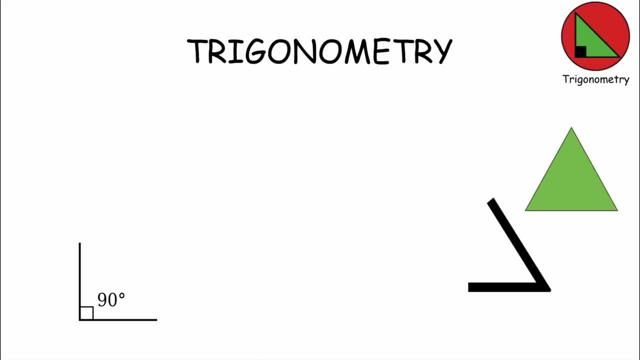 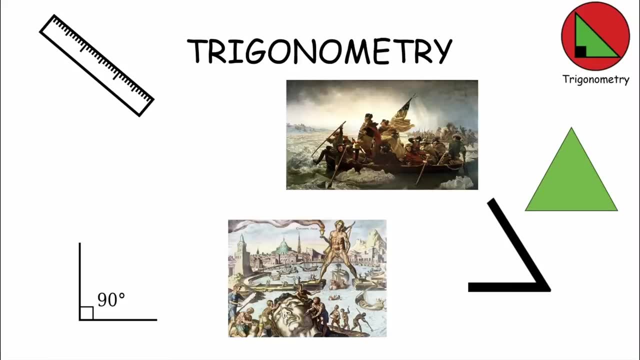 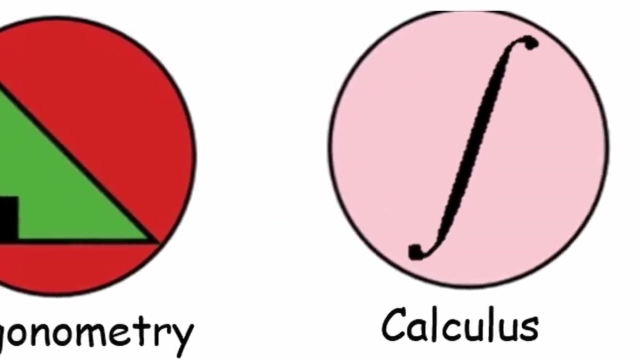 It helps us understand and calculate things like distances, heights and angles in various situations, such as in navigation, architecture and physics. Trigonometry uses functions like sine, cosine and tangent to solve these triangle-related problems. Calculus- Calculus is a type of math that deals with changes and motion. 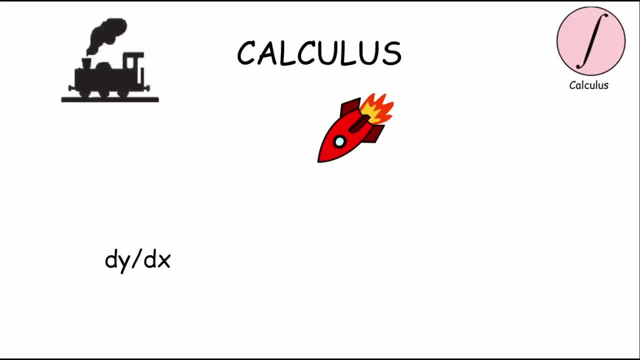 Calculus involves concepts like derivatives, which describe rates of change and go from distance to speed to acceleration. Integrals or antiderivatives do the opposite and help us find the total amount of change Statistics- Statistics is a branch of math that involves collecting, organizing and interpreting data to make informed decisions. 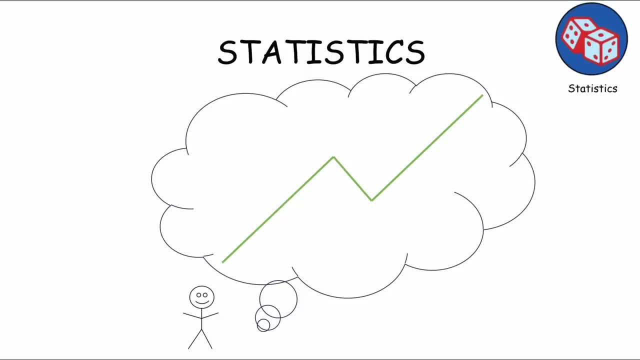 It helps us understand and describe the world around us. It helps us understand and describe patterns in information, such as averages, trends and probabilities. Statistics is used in various fields like sports, science and business to draw meaningful conclusions from data. 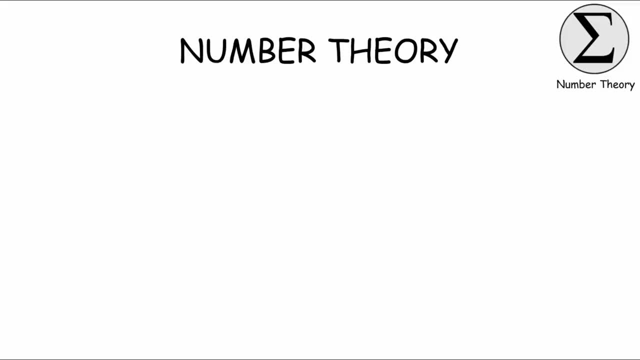 Number Theory. Number theory is a branch of mathematics that explores the properties and relationships of whole numbers like 1,, 2, and 3.. Number Theory is a branch of mathematics that explores the properties and relationships of whole numbers like 1,, 2, and 3.. 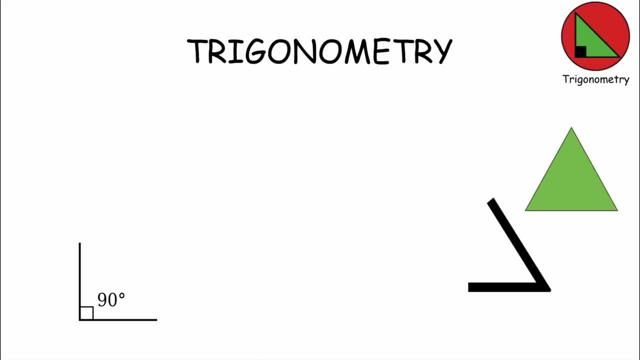 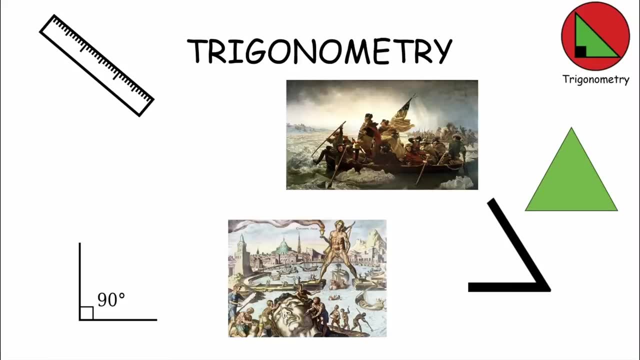 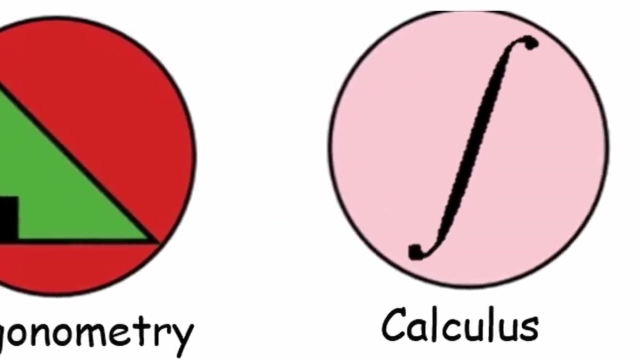 It helps us understand and calculate things like distances, heights and angles in various situations, such as in navigation, architecture and physics. Trigonometry uses functions like sine, cosine and tangent to solve these triangle-related problems. Calculus- Calculus is a type of math that deals with changes and motion. 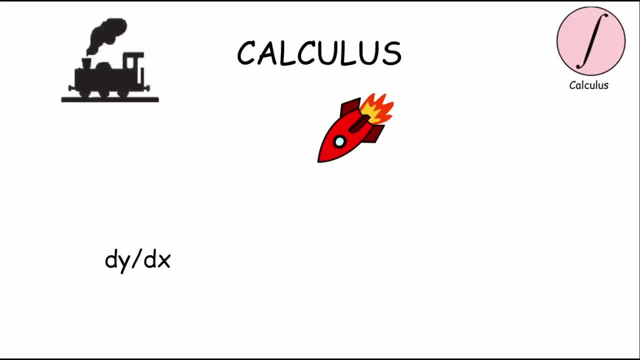 Calculus involves concepts like derivatives, which describe rates of change and go from distance to speed to acceleration. Integrals or antiderivatives do the opposite and help us find the total amount of change Statistics- Statistics is a branch of math that involves collecting, organizing and interpreting data to make informed decisions. 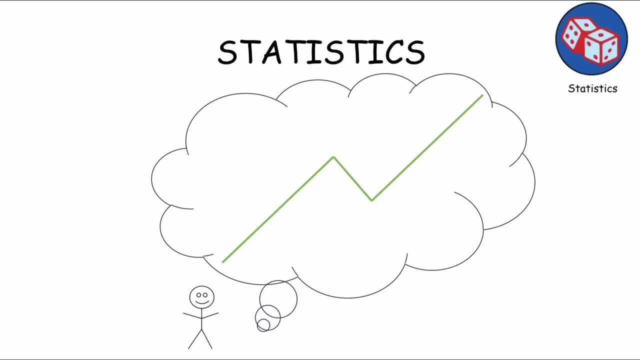 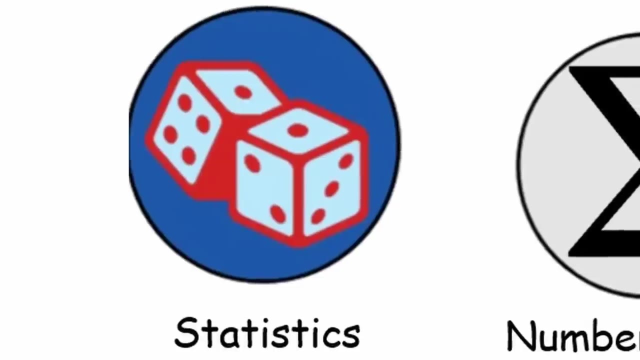 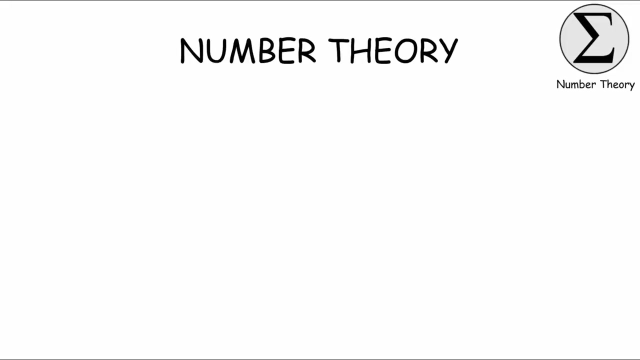 It helps us understand and understand the situation, patterns and information such as averages, trends and probabilities. statistics is used in various fields like sports, science and business to draw meaningful conclusions from data. number theory- number theory is a branch of mathematics that explores the properties and relationships of whole numbers, like 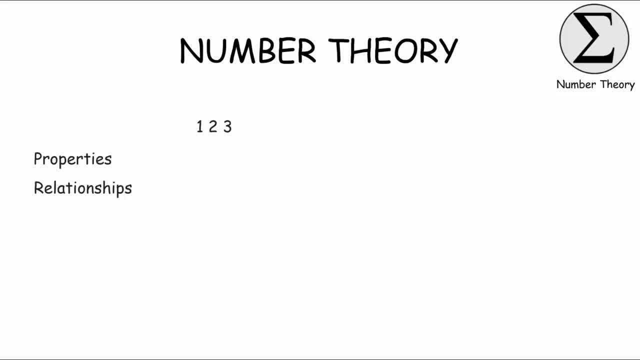 one, two and three. it involves studying patterns and properties of numbers to understand their behavior. number theory is often like solving puzzles with whole numbers, looking for interesting and unique ways these numbers interact with each other. a simple example of number theory is the pattern in prime numbers of the tendency for prime gaps to become larger as we examine larger prime. 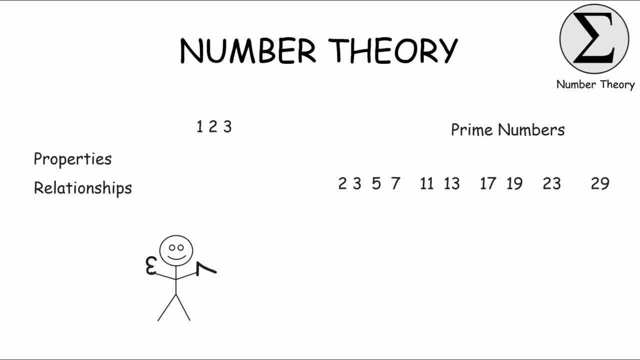 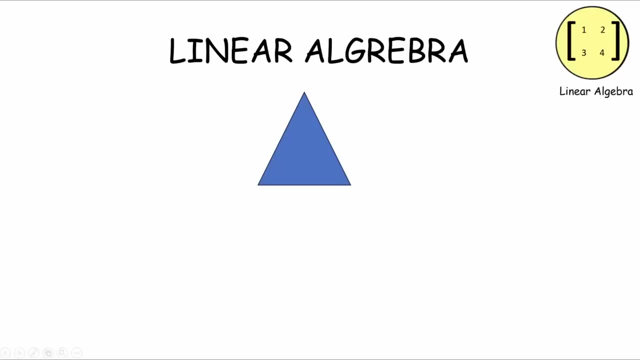 numbers. prime gaps refer to the difference between consecutive numbers and the tendency for prime gaps to become larger. consecutive prime numbers. while there is no predictable formula for the exact gap size, number theory helps us explain why, on average, the gaps tend to get larger as we look at higher prime numbers. linear algebra- linear algebra is: 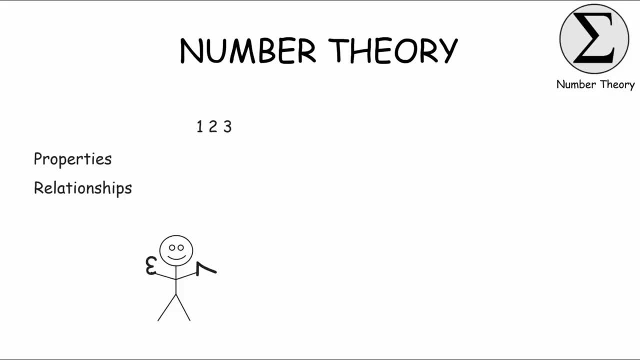 It involves studying patterns and properties of numbers to understand their behavior. Number Theory is often like solving puzzles with whole numbers, looking for interesting and unique ways these numbers interact with each other. A simple example of Number Theory is the pattern in prime numbers of the tendency for prime gaps to become larger as we examine larger prime numbers. 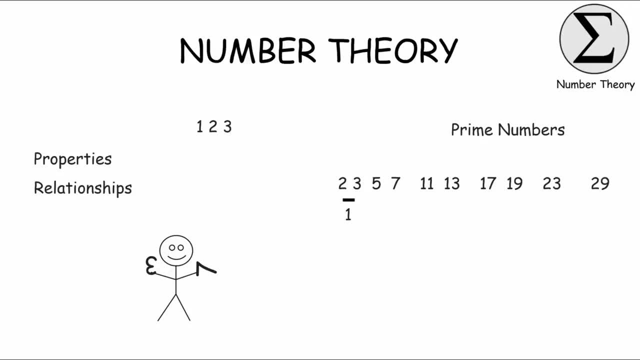 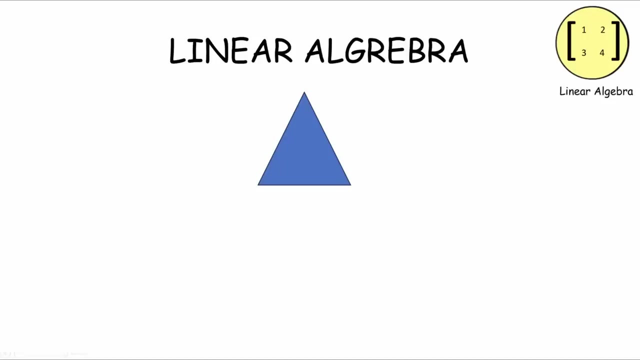 Prime gaps refer to the difference between consecutive prime numbers. while there is no predictable formula for the exact gap size, Number Theory helps us explain why, on average, the gaps tend to get larger as we look higher prime numbers. Linear Algebra- Linear Algebra- Linear Algebra is a branch of mathematics that deals with lines, planes and spaces using equations and matrices. 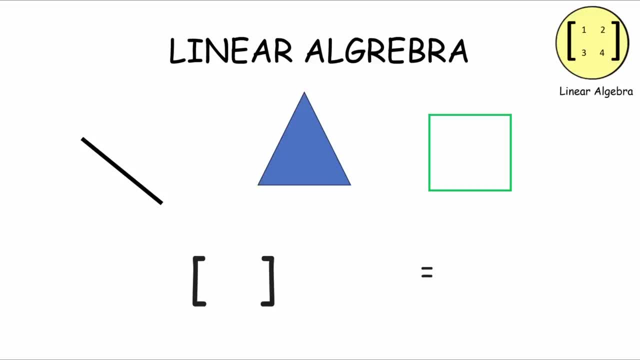 Linear Algebra is a branch of mathematics that deals with lines, planes and spaces using equations and matrices. Linear Algebra is a branch of mathematics that deals with lines, planes and spaces using equations and matrices. It helps us solve systems of equations and understand transformations like stretching. 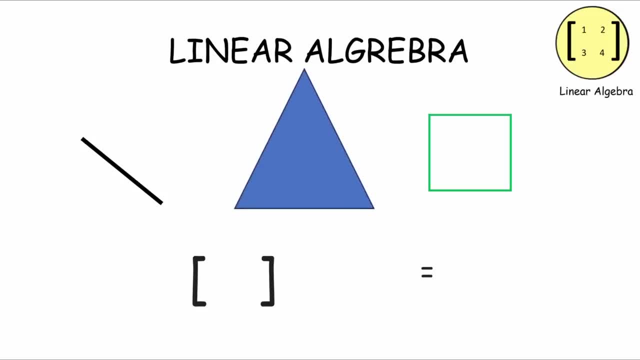 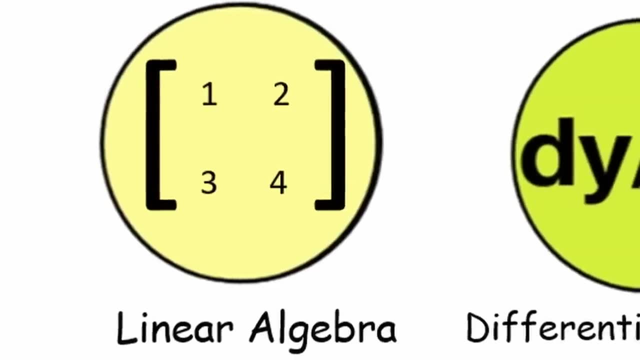 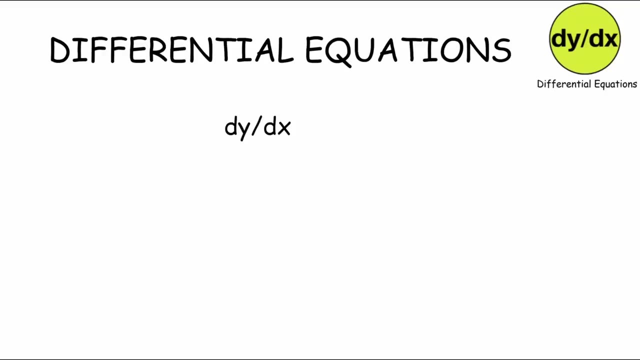 or rotating shapes. Linear algebra is like a toolset for working with multiple variables and relationships in a coordinated way. Differential Equations- Differential equations- are a type of calculus that helps us understand how things change. They involve rates of change and show how a quantity depends on its own rate of change. 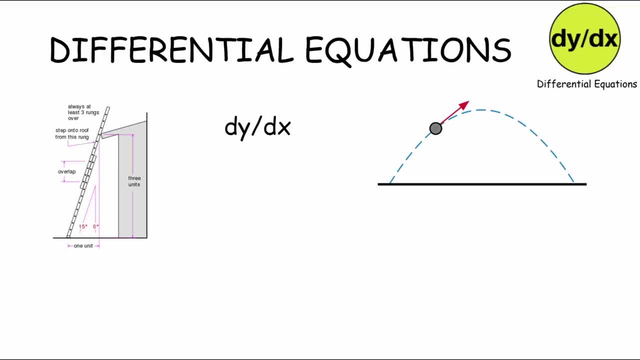 The falling ladder problem is a classic example of a differential equation in physics. Imagine a ladder leaning against a wall and sliding down. The angle between the ladder and the ground changes as it falls. You can use this equation to figure out the speed the ladder falls at. 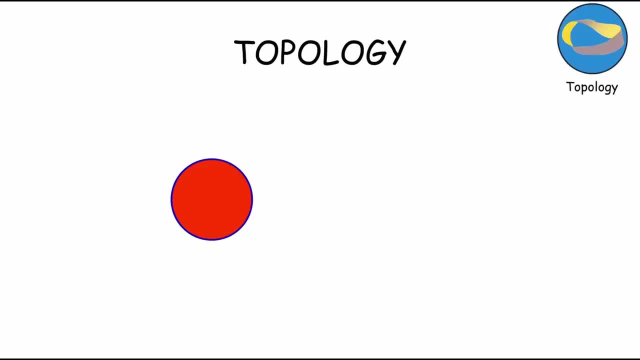 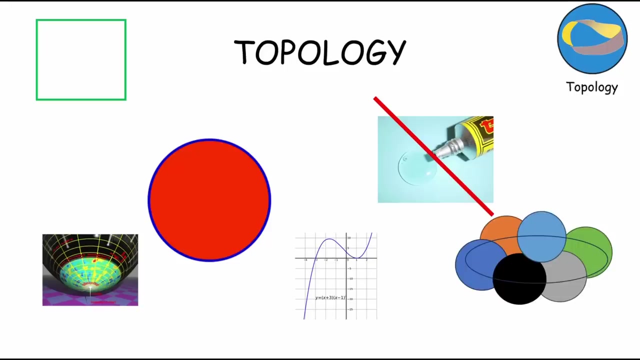 Topology- Topology. Topology is a branch of mathematics that deals with the properties of space that are preserved under continuous deformations, such as stretching, crumbling and bending, but not tearing or gluing. Topology often includes the study of open sets, continuity, compactness and various 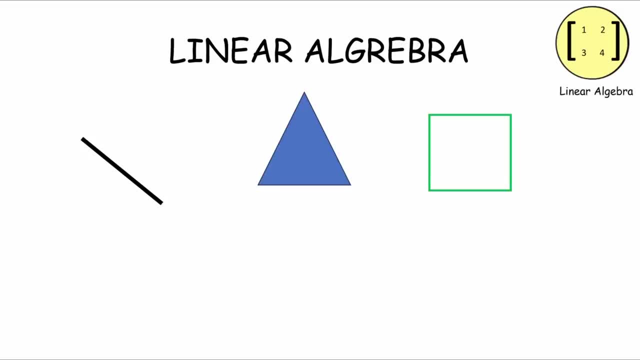 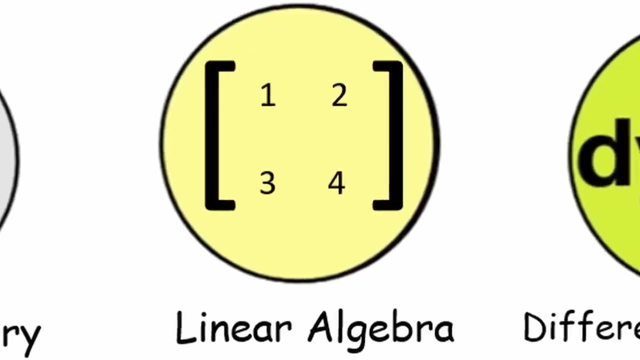 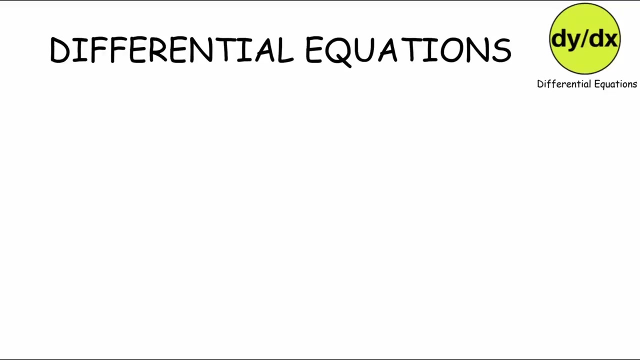 a branch of mathematics that deals with lines, planes and spaces using equations and matrices. it helps us solve systems of equations and understand transformations like stretching or rotating shapes. linear algebra is like a toolset for working with multiple variables and relationships in a coordinated way. differential equations: differential equations- are a type of calculus that 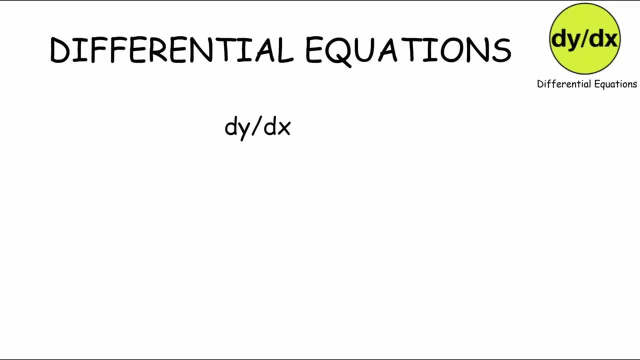 helps us understand how things change. they involve rates of change and and show how a quantity depends on its own rate of change. the following ladder problem is a classic example of a differential equation in physics. imagine a ladder leaning against a wall and sliding down the angle between the 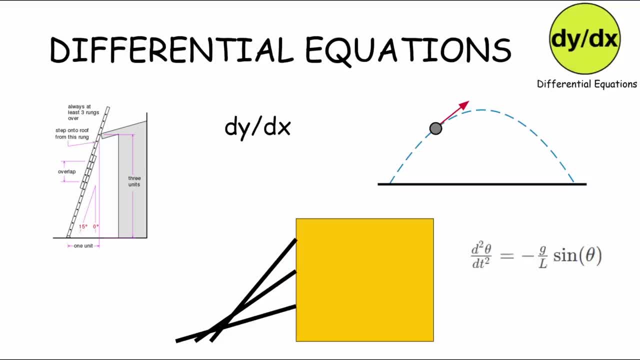 ladder and the ground changes as it falls. you can use this equation to figure out the speed the ladder falls at topology. topology is a branch of gravity. making responses to eat them faster at the center level are called vertical side Equalities. we know is stage and g schools that our theories measure amazing. 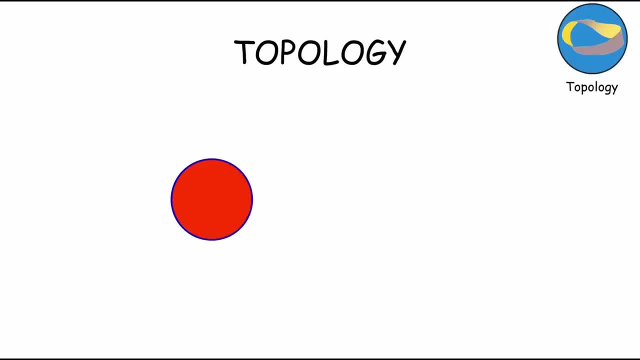 velocity energy, 하기 in th手 like this, the word ge accelerator might even be at safer and natural yet. otherwise we won't be able to grasp again. if there were any things we would know, put them both themselves, but we'd prefer to work on more Conänder's. 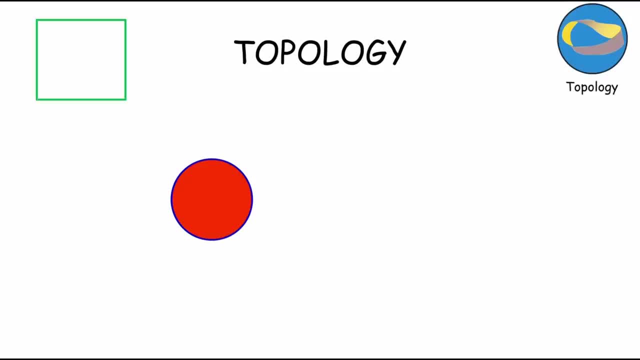 of mathematics that deals with the properties of space that are preserved under continuous deformations such as stretching, crumbling and bending but not tearing or gluing. Topology often includes the study of open sets, continuity, compactness and various topological structures like manifolds. 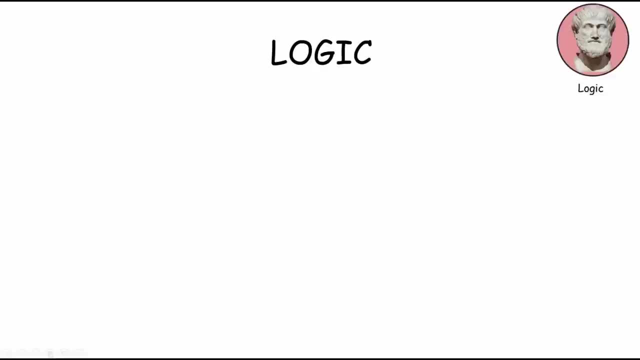 Logic. Logic in math is a set of rules that helps us figure out what is true or false based on reasoning. It involves making clear and sensible arguments using statements that are either true or false, and understanding how different statements relate to each other. Logic helps us make sure our math conclusions 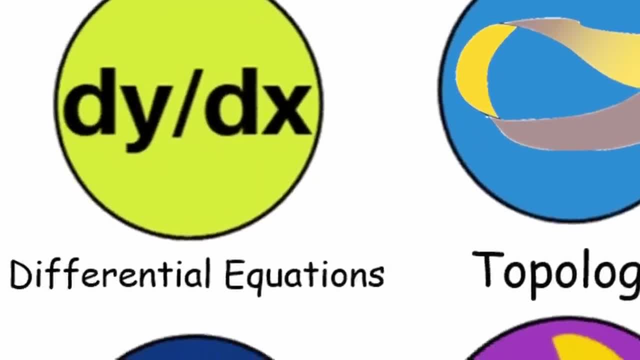 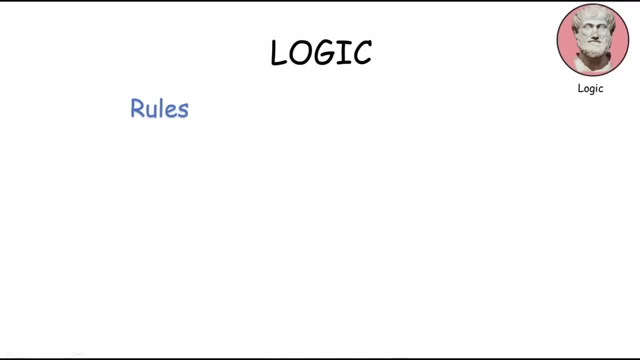 topological structures like manifolds, Logic, Logic and math. Topology and math. Topology and math. Math is a set of rules that helps us figure out what is true or false based on reasoning. It involves making clear and sensible arguments using statements that are either true or false. 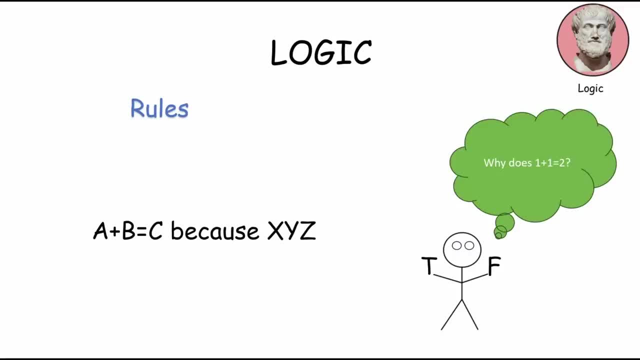 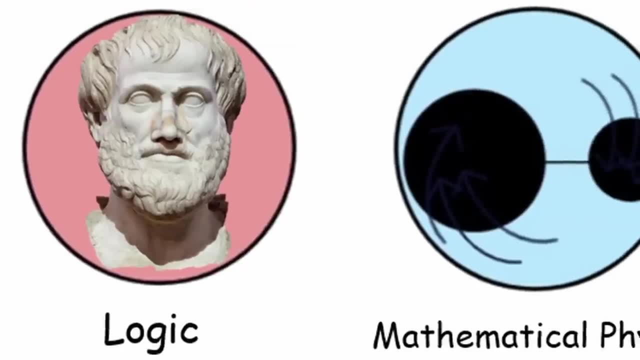 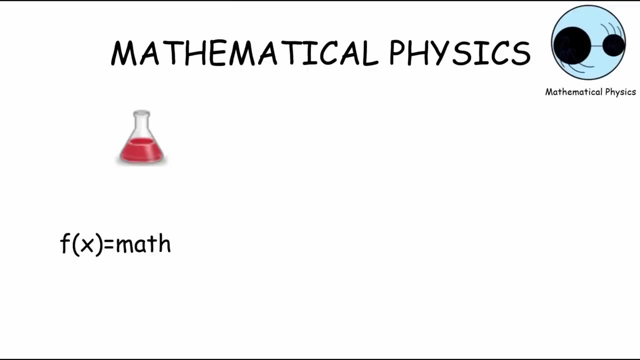 and understanding how different statements relate to each other. Logic helps us make sure our math conclusions are sound and reliable. Mathematical Physics. Mathematical physics is a branch of mathematics, that is, a branch of science, where math is used to describe and understand the fundamental principles of the physical world. 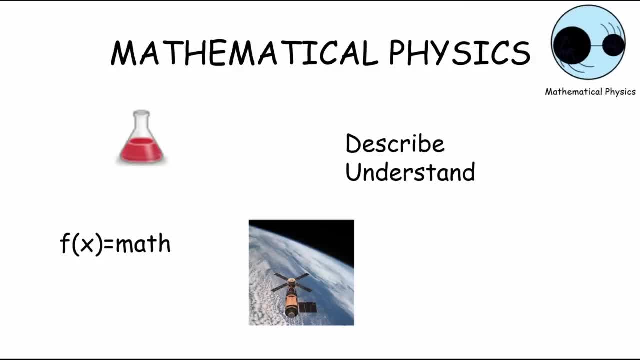 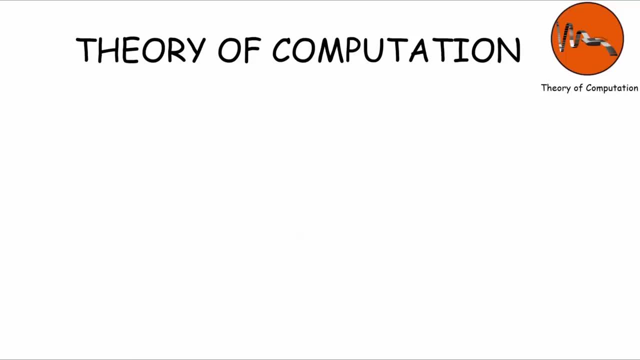 Scientists use mathematical equations and models to explore phenomena like motion, electricity and light. Theory of Computation. The theory of computation is a set of ideas that help us understand what computers can and cannot do. It explores how problems can be solved using the computer. 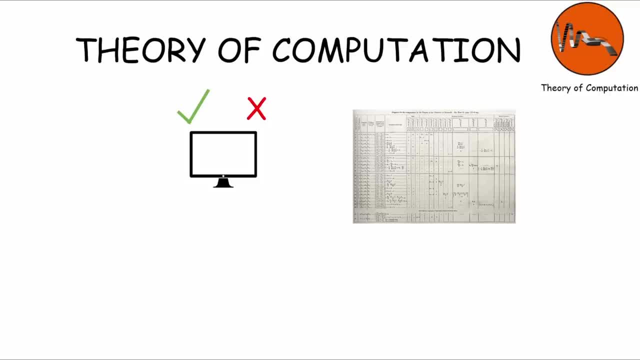 The theory of computation is a set of ideas that help us understand what computers can and cannot do. It explores how problems can be solved using the computer. The theory of computing- The theory of computing System ofесks Sounds like tempo Using algorithms, which are step-by-step instructions and look at the limits of what can be achieved. 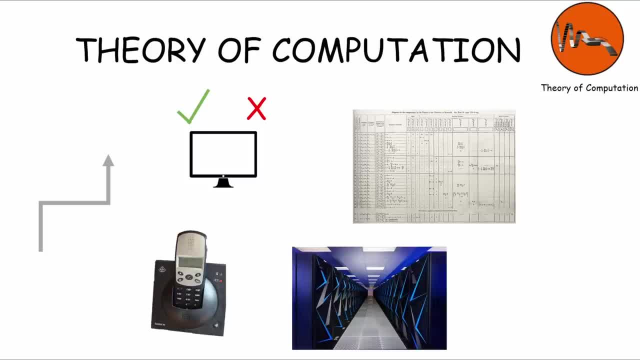 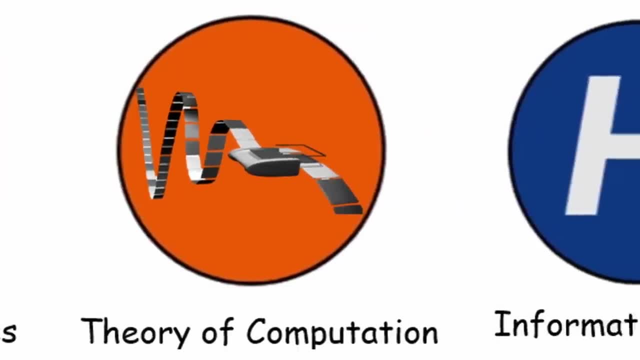 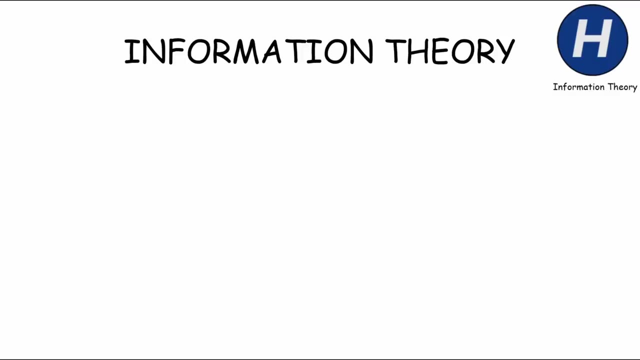 with different types of computing devices. It's like figuring out the rules and possibilities of how computers work and what they're capable of influence. How To Use Smart Computing. 1. Information Theory. 1. Information theory is a branch of study that focuses on how information is transmitted. 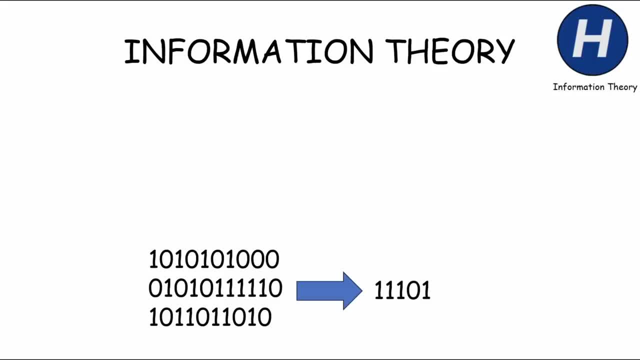 and processed. It helps us measure and understand how something works. 2. measure and understand the amount of information in a message, considering concepts like data comprehension. In simpler terms, it's like exploring the best way to send and receive information. An easy example of information theory is thinking about sending a message. 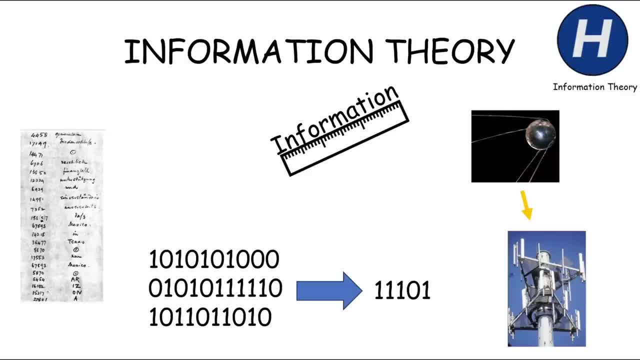 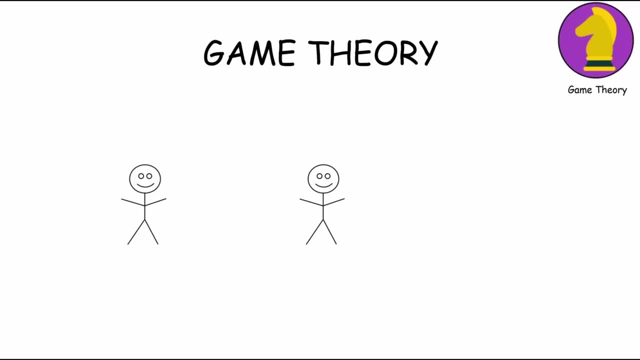 in secret code. Information theory helps us measure how much information is stored in the coded message and how efficiently it can be transmitted. Game theory: Game theory is like a way of thinking about how people make decisions when they interact with each other. It helps us. 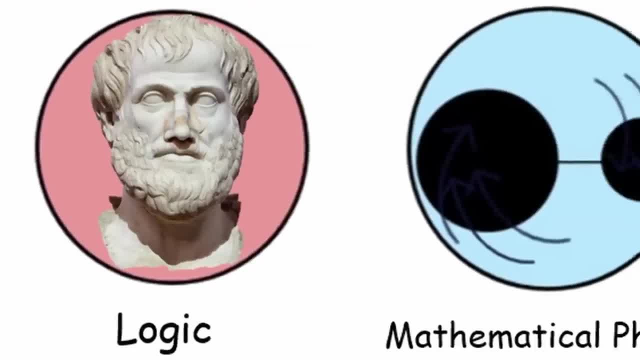 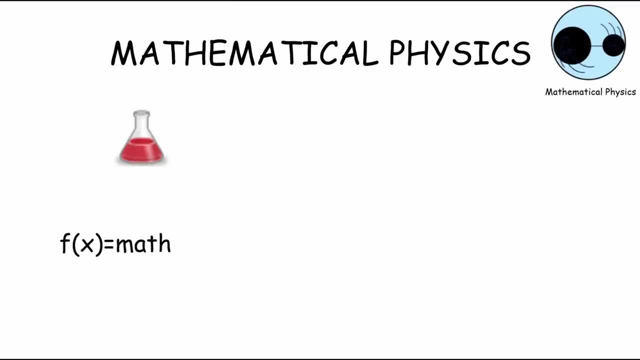 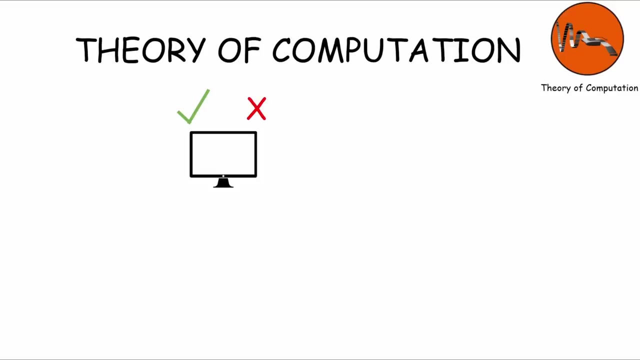 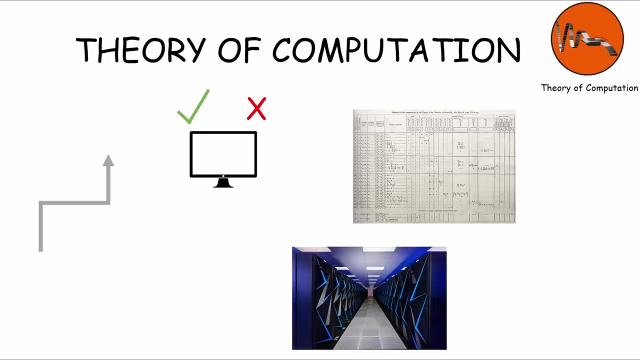 are sound and reliable. Mathematics. Mathematical physics. Mathematical physics is a branch of science where math is used to describe and understand the fundamental principles of the physical world. Scientists use mathematical equations and models to explore phenomena like motion, electricity and light. Theory of computation. The theory of computation is a set of ideas that help us understand what computers can and cannot do. It explores how problems can be solved using algorithms, which are step-by-step instructions, and look at the limits of what can be achieved with different types of computational devices. 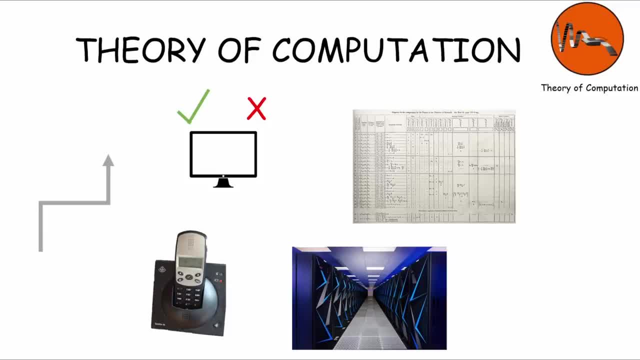 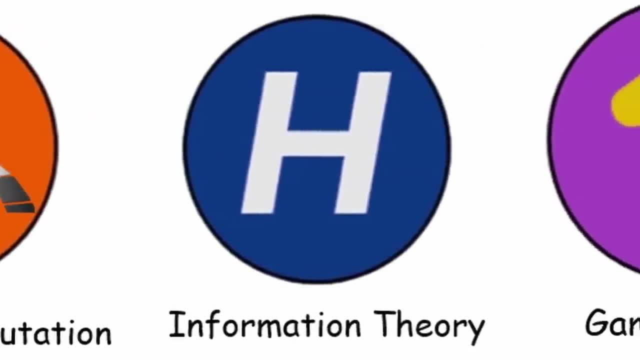 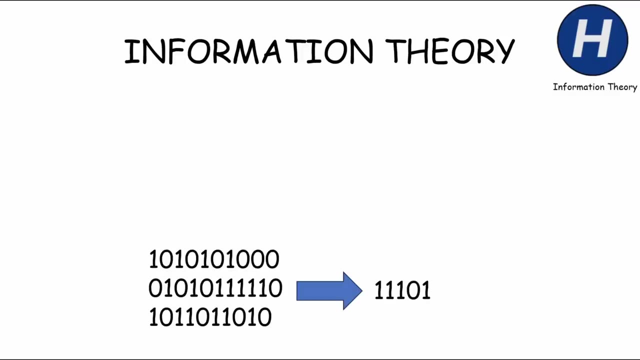 It's like figuring out the rules and possibilities of how computers work and what they're capable of. Information theory: Information theory is a branch of study that focuses on how information is transmitted and processed. It helps us measure and understand the amount of information in a message, considering concepts like data comprehension. 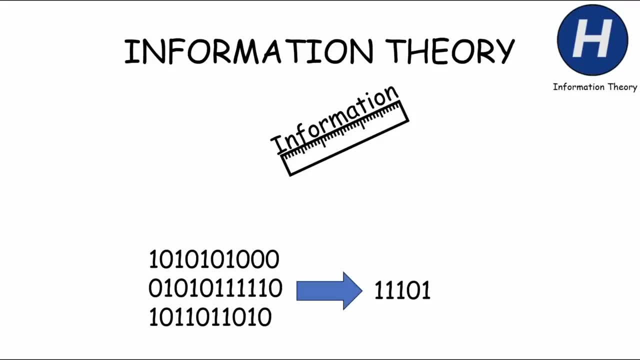 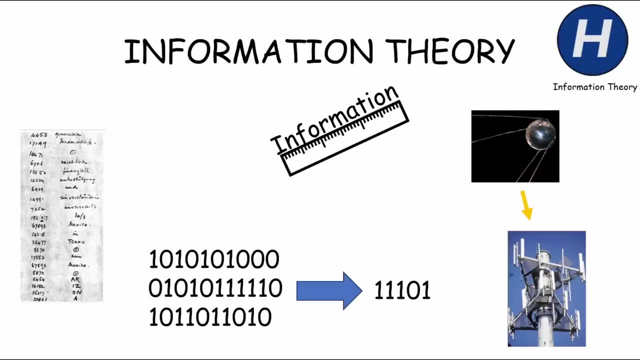 In simpler terms, it's like exploring the best way to send and receive information. An easy example of information theory is thinking about science Sending a message in secret code. Information theory helps us measure how much information is stored in the coded message and how efficiently it can be transmitted. 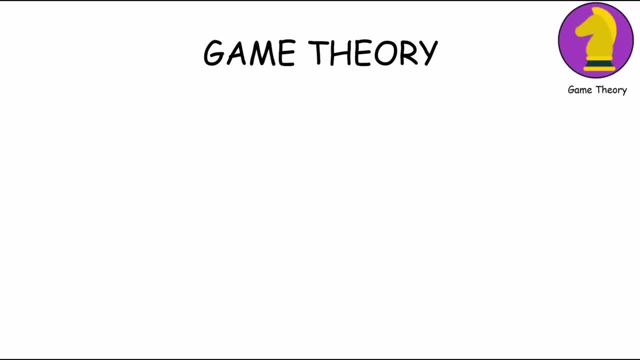 Game theory. Game theory is like a way of thinking about how people make decisions when they interact with each other. It helps us understand strategic thinking and choices in situations where what one person decides Can affect what others should do. An example of game theory is the prisoner's dilemma. 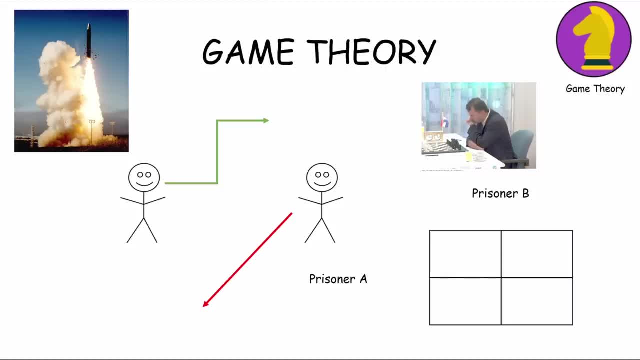 Two individuals are arrested and accused of a crime. They are held in separate cells and cannot communicate. The authorities offer each prisoner a deal: If one stays silent while the other confesses, the one who confesses gets a reduced sentence and the one who stays silent gets a harsher sentence. 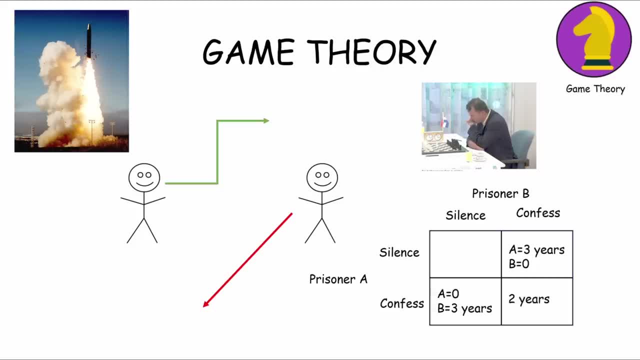 If both confess, the one who confesses gets a reduced sentence and the one who stays silent gets a harsher sentence. If both confesses, the one who confesses gets a reduced sentence. In other words, if two people confess, they receive moderate sentences.